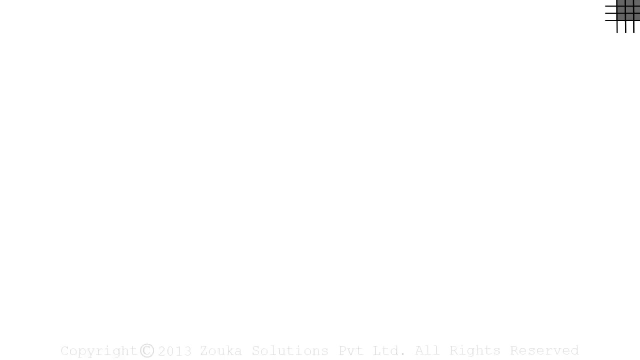 Understanding how the surface area of a cylinder is derived is very interesting. Look at this cylinder. It has two blue circular ends, one on top and one at the bottom. Analyze the figure. As we know the area of a circle, we can easily find the surface area. 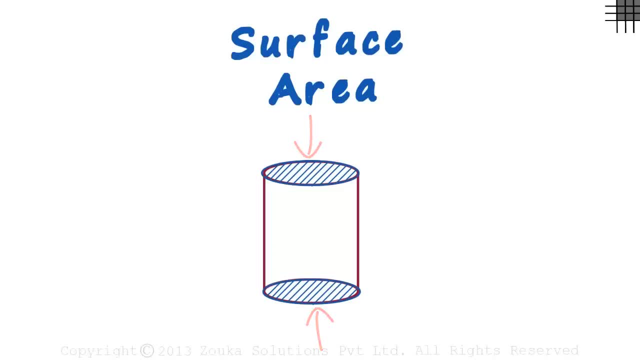 of the top and the bottom circular ends. But the important question is: how do we find the surface area of this curved surface? Let's zoom out a bit. First, let's separate the circular ends: This is the top one and this is the one at the bottom. To understand, 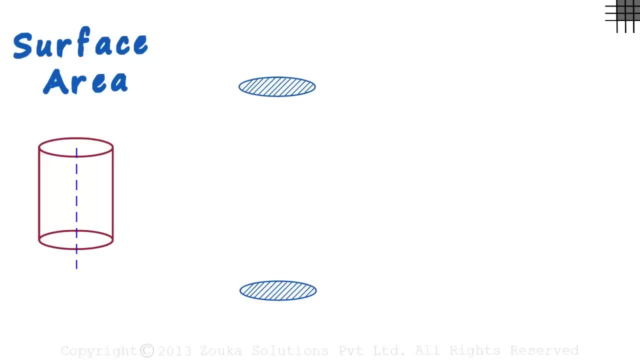 the curved surface. we cut it open vertically, which will make it look like this: We just cut the surface vertically. When this is opened up further, it will look like a rectangle. There are a few other ways to cut a curved surface. For example, we can cut a cylinder. 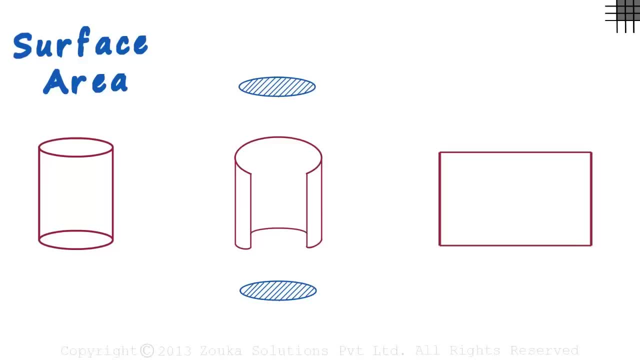 like this. The large surface of this cylinder will look like this: First, what is the length of the rectangle And second, what is it's breadth. If you look carefully, you will notice that the length of this rectangle is actually the circumference. 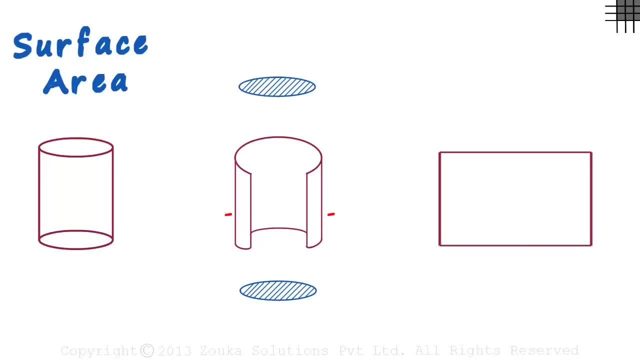 of the circular base, Because all we did was pull this open. What about its breadth? Its breadth is the height of the cylinder. Let's assume the height of the cylinder is: let's cylinder is h and the radius of the circular base is r. 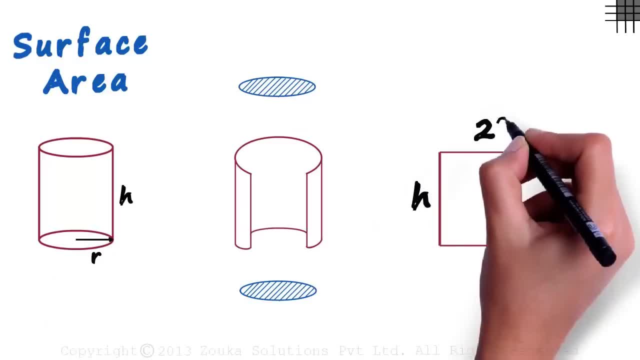 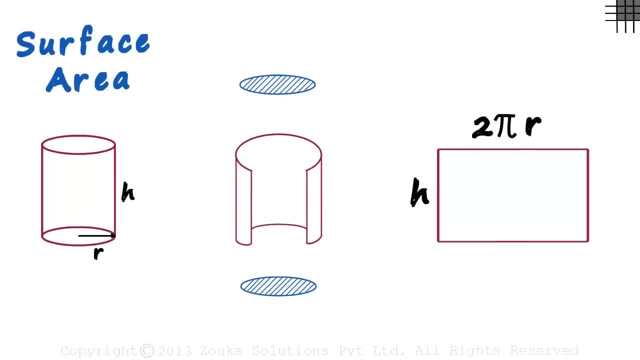 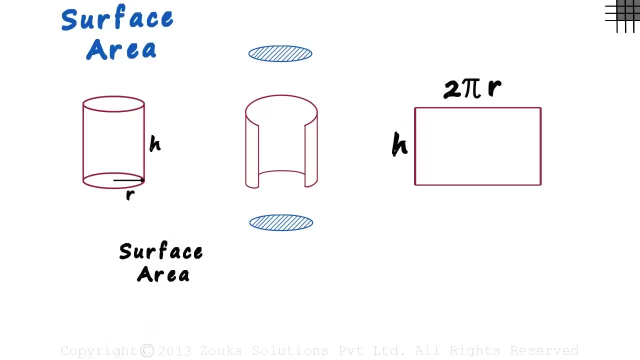 So the breadth will be h and the length will be 2 pi r. Don't forget, the area of this rectangle will be the curved surface area, But we need to find the total surface area of this cylinder. The surface area will be the sum of all these three surfaces. 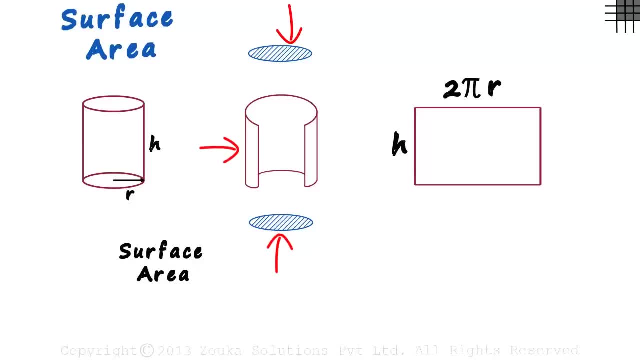 Two circles and the curved surface, which is the rectangle. The area of the circular base is pi r squared. Since there are two equal circles, we write pi r squared plus pi r squared. This covers the surface area of the top and the bottom surfaces.